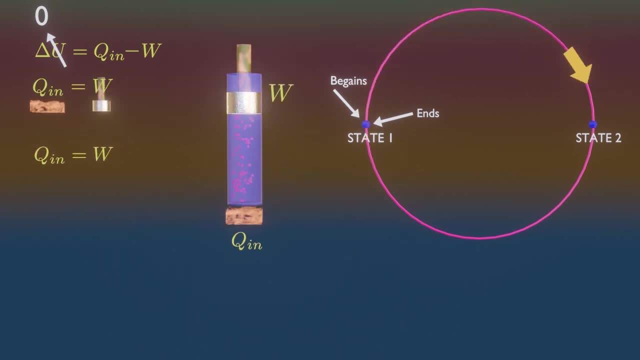 If somehow it was able to operate on cycle without rejecting any heat, then every heat is converted to work. There is no heat loss and it violates second law. This types of device is called a perpetual motion machine. It do not exist in real life. 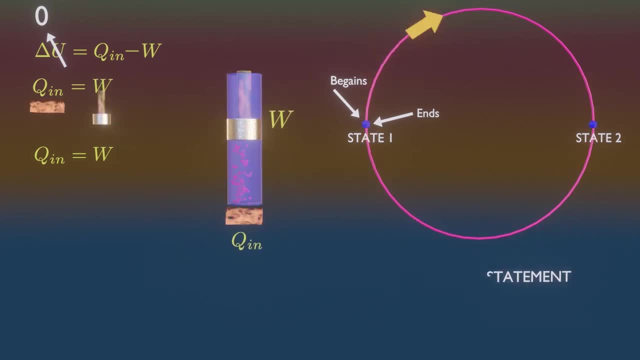 The Calvin-Planck statement of second law tells us about the same thing, about this thermodynamic cycle. It says that it is impossible for any device that operates on a cycle to receive heat from a single reservoir and provide net amount of work. 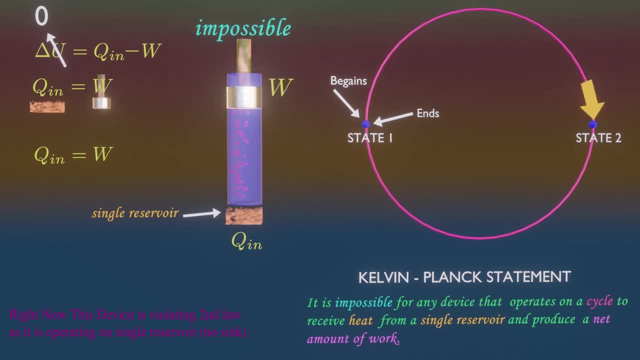 This device is operating on cycle, receiving heat from single reservoir and producing the net amount of work. So if 100 kilojoules of heat it received, then 100 kilojoules of work is done during cycle. It has thermal efficiency of 100%. 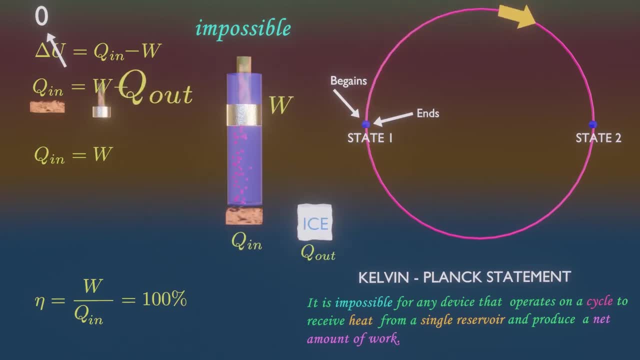 But our statement of second law tells us that it must reject heat in order to operate on cycle. So the gas inside the cylinder must exchange heat with the cold environment as well as the heat source, And it can never achieve 100% thermal efficiency. 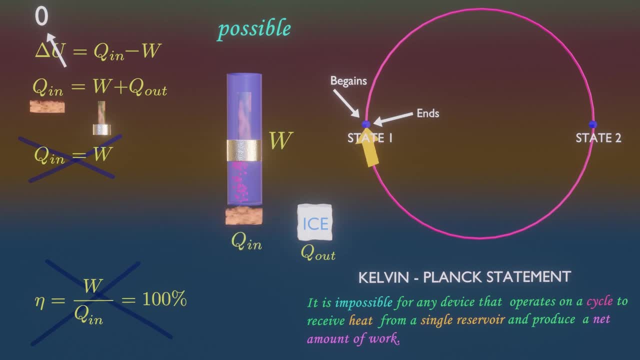 And also, it is true, even under idealized condition, This device won't get 100% efficiency, even if you assume an ideal gas as a working fluid and a frictionless piston. That's what second law says. The impossibility of having a 100% efficient heat engine is not due to friction or other dissipative effects. 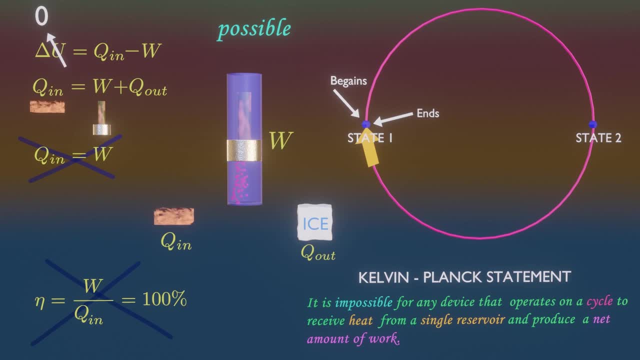 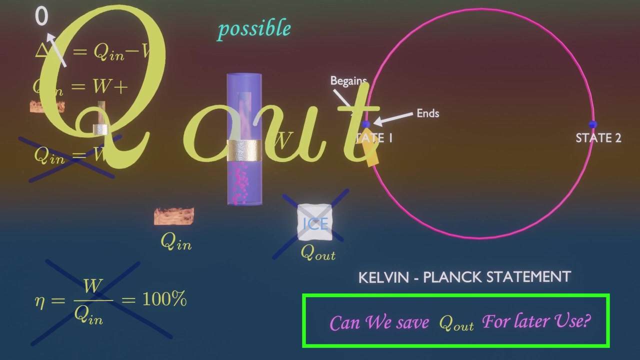 It is a limitation that applies to both the idealized and the actual heat engines. Now let us try to conserve this waste heat for later use. If it is conserved, then we don't need sink or condenser to reject heat. 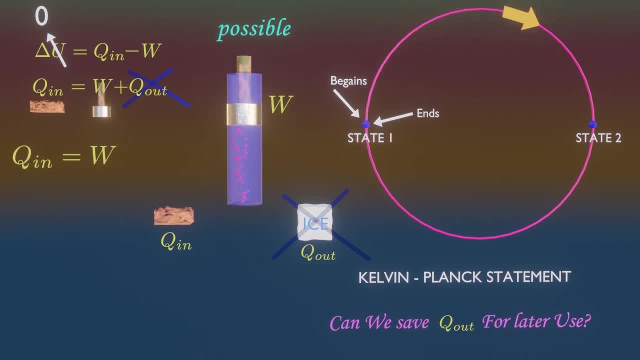 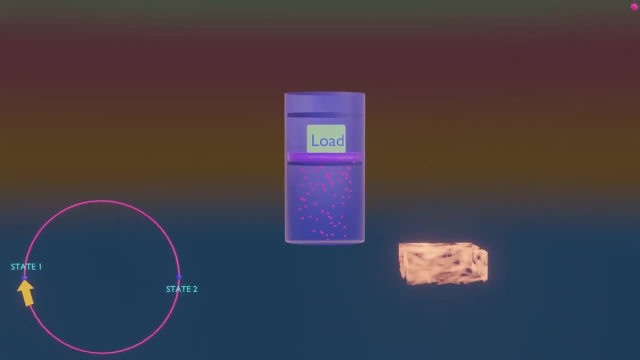 And every heat given is converted to work for any cyclic process. Let us consider a simple heat engine that is used to lift weight. A heat engine is a device that convert heat to work and it operates on cycle. Assume the working fluid inside this heat engine as an ideal one. 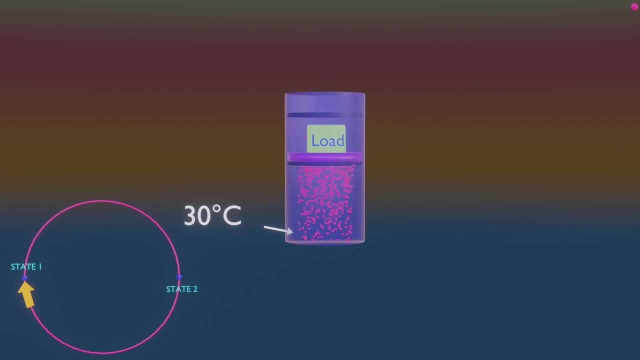 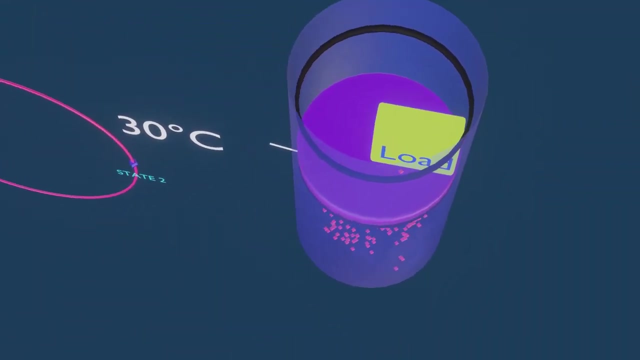 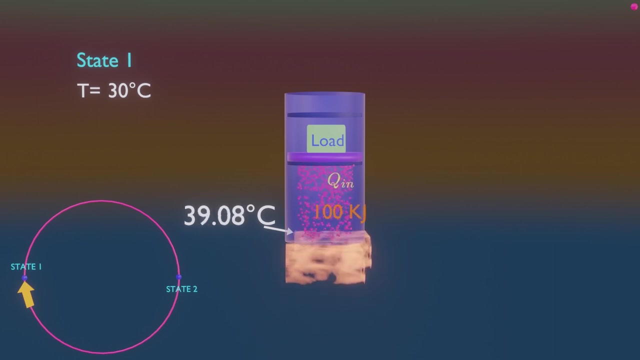 Initially the gas temperature is 30°C. The piston which is loaded with the weights is resting on top of the lower stops. Now 100 kJ of heat is given to the piston, Then to this gas from the source at 100°C, causing it to expand and to raise the loaded piston until the piston raises the upper stops. 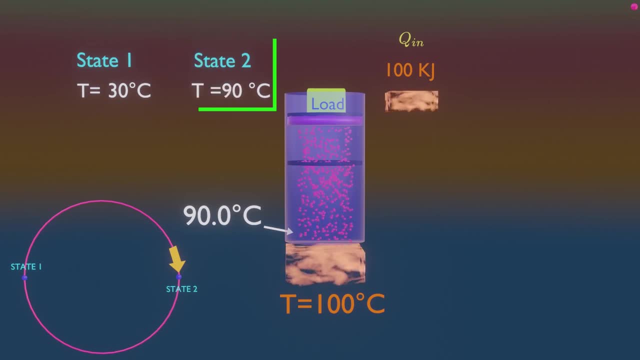 At this point our heat engine is in state 2. Here the load is removed and the gas temperature is observed to be 90°C. The work done on the load during this expansion is equal to the increase in its potential energy, say 40 kJ. 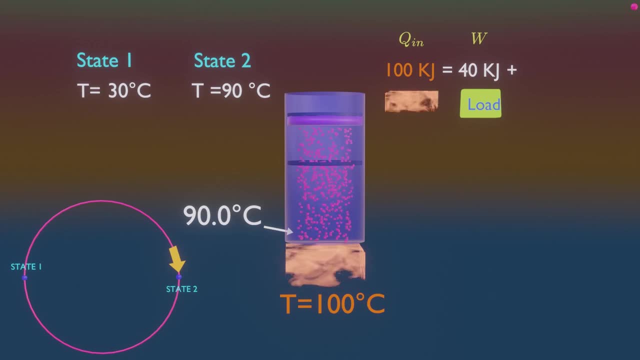 Look, even under ideal condition, the amount of heat supplied to the gas is greater than work done. Now it raised the questions About what happened To other 60 kJ of energy. According to first law energy conservation, This extra energy is used to increase the change in internal energy of gas. 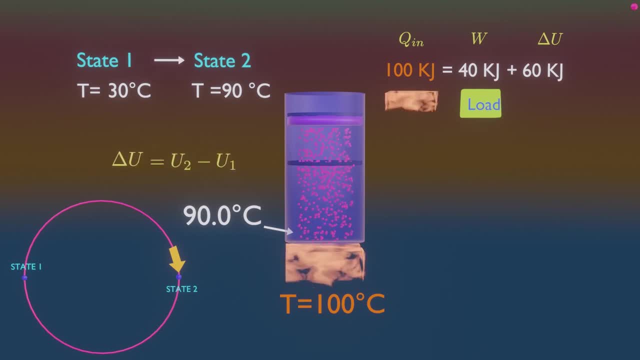 Which is change of energy from state 1 to state 2.. But you know, for an ideal gas, internal energy is function of temperature. only Do you know what this mean? It means that some part of heat energy is used to raise the temperature of gas. 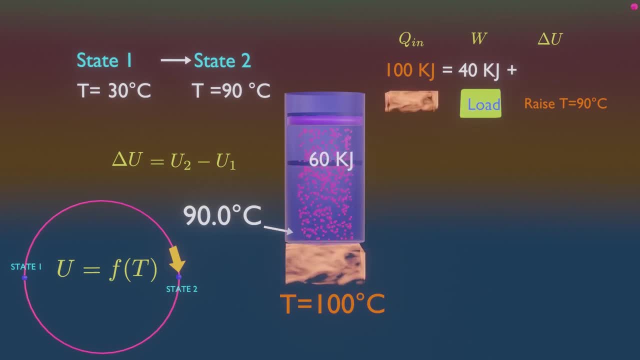 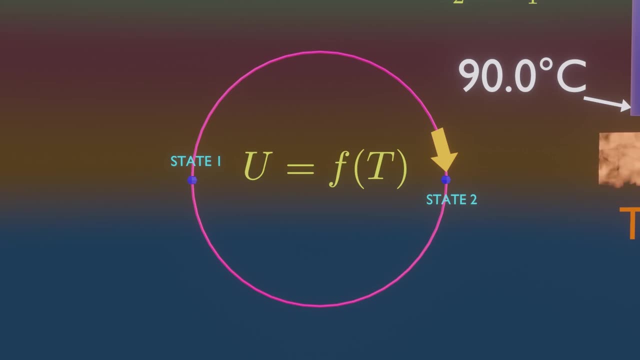 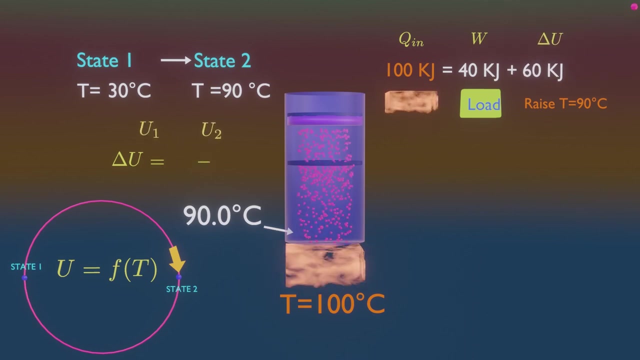 In this case 60 kJ of heat energy is used to raise the temperature. Also, remember, only half the cycle is complete here. So change in internal energy from state 1 to state 2, is not zero. It sucks some of heat energy to raise the temperature of gas. 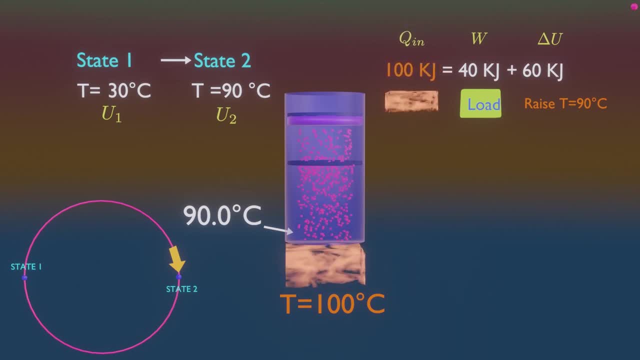 So with 100 kJ of heat given, only 40 kJ is used to do work And remaining 60 kJ of energy is used to increase the temperature of gas. Now let us try to answer this question: Is it possible to transfer the 60 kJ of excess heat at 90°C back to the reservoir at 100°C for later use? 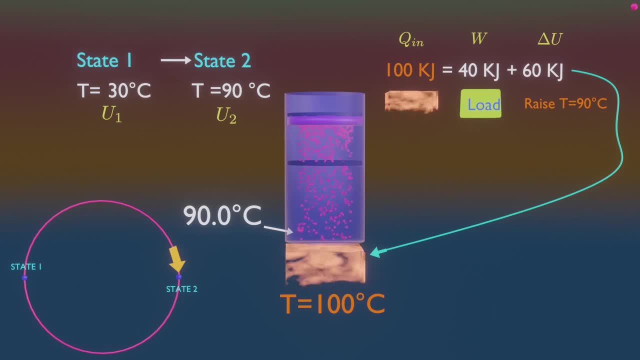 I mean cooling this gas from 90°C to 30°C by conserving this 60 kJ of heat and returning to initial state and complete the cycle. Well, this question can be solved, But we need both first and second law for this. 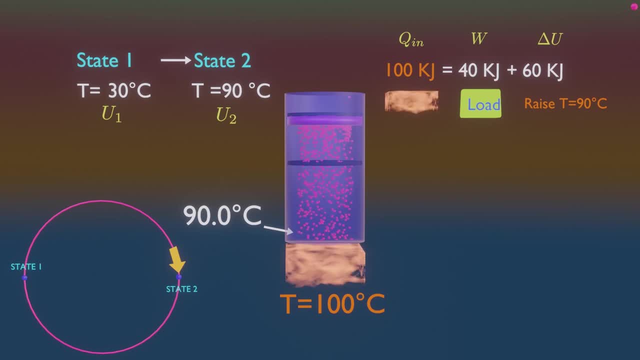 You know, in this case, In cyclic process, change in internal energy is zero and according to first law, only every heat must be converted to work, But according to second law that is impossible. Some energy must be rejected to colder body in order to operate on cycle. 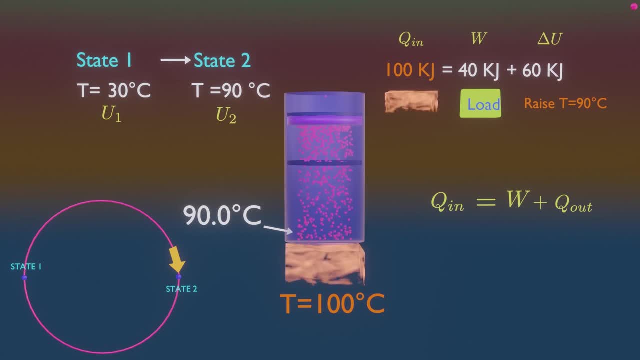 So if you follow second law, you can't conserve this energy. This waste heat must be rejected to colder body And on cyclic process. this heat engine has thermal efficiency of 40%. But if you do not follow second law and follow first law only, 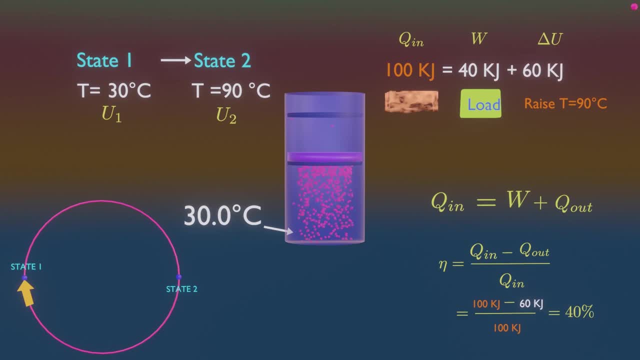 Then you can conserve this excess heat, Because first law is still valid, if you assume that heat can reverse its direction And can travel from lower temperature to higher temperature and complete the cycle. So if this gas is cooled back to initial state by transferring heat back to hotter body,